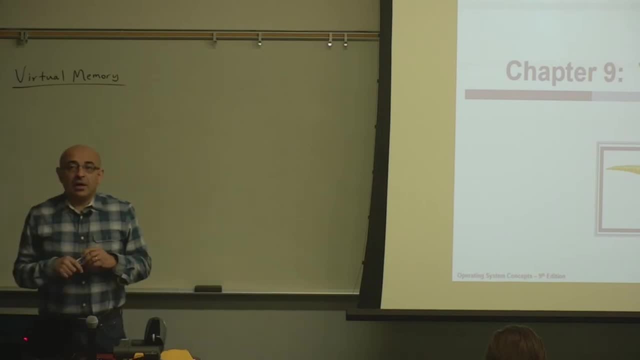 with contiguous memory allocation and the alternative methods, the non-contiguous memory allocation techniques. So what was the main problem with contiguous memory allocation? Yeah, fragmentation, exactly. So we looked into contiguous memory allocation and we realized that the main problem was that it causes a serious problem, which is fragmentation. because insisting on finding a whole contiguous chunk of memory for each program doesn't give the memory management system enough flexibility to utilize existing memory. You may have, memory may be available, there may be free memory available, but it's just not contiguous. We don't have that contiguous chunk of memory that we need. 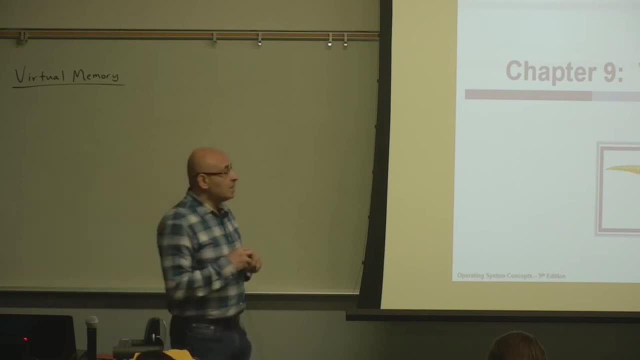 So contiguous memory allocation is not a good idea. So that's why people came up with the ideas of segmentation and paging. And in segmentation and paging you divide the address space of a process into pieces that you call segments or pages, and then you do segmentation. 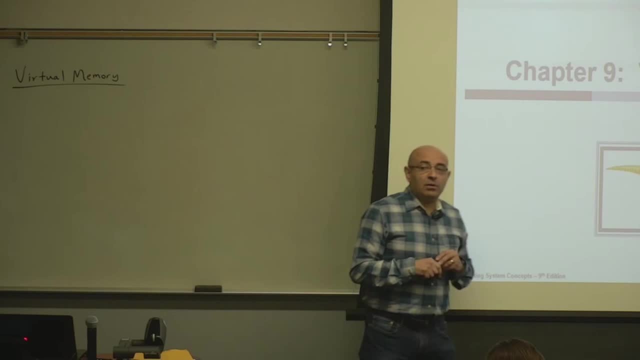 So you divide the memory allocation at the segment level or at the page level, And that gives the system a lot more flexibility. It makes it much easier to utilize the free memory that is available Now. in the previous chapter we introduced the notion. 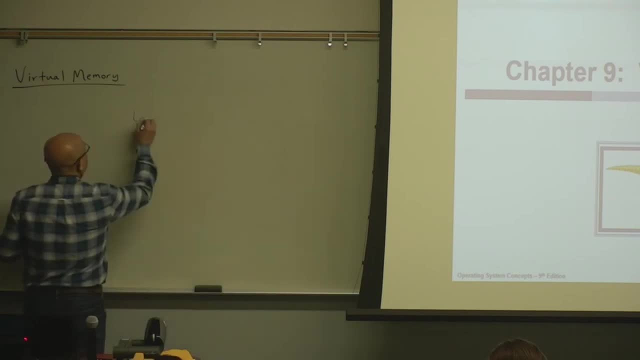 of the logical address space- Logical address space of a process- and the physical address space, And the main point is that in the logical address space you have a contiguous piece of memory that consists of pages, But physically, in physical memory, these pages may be scattered all over the memory. 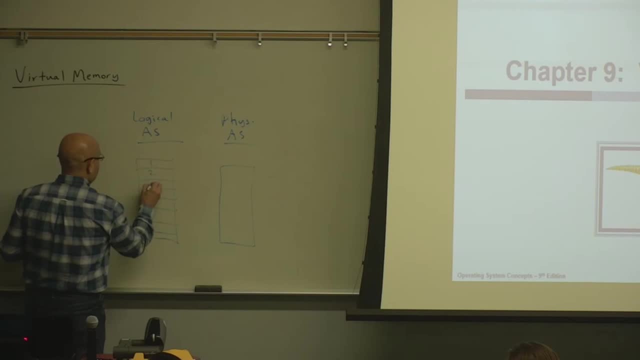 So they don't have to be. So. this is page one, page two, page three. So page one may be here, page two may be here and page three may be here, So they don't have to be adjacent in physical memory. 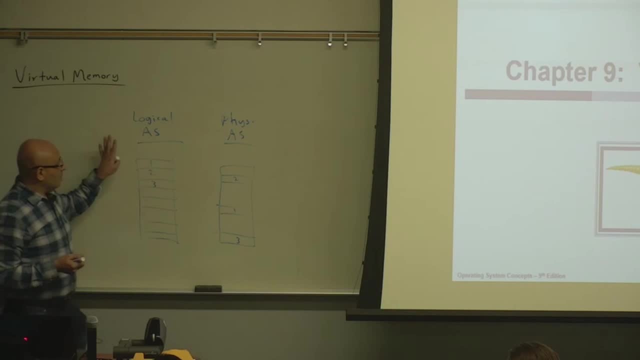 and they don't have to be in order. So that was the. you know the concept of the logical address space and the physical address space. Logically, memory looks contiguous. If you have a big array in your program, it's going to look contiguous to you. 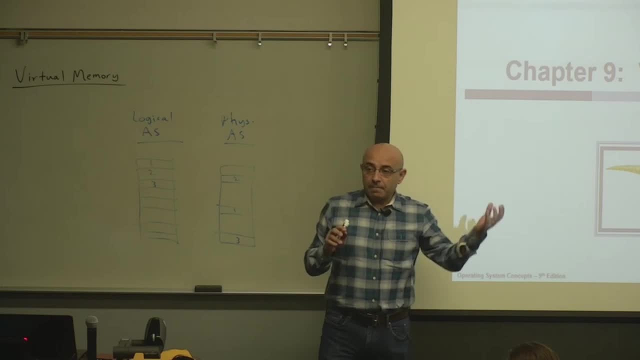 For you, that array is contiguous, even though physically it may be scattered all over memory. Now, with virtual memory, the difference between logical and physical is going to be even bigger. The key idea in virtual memory is that when a program is running, 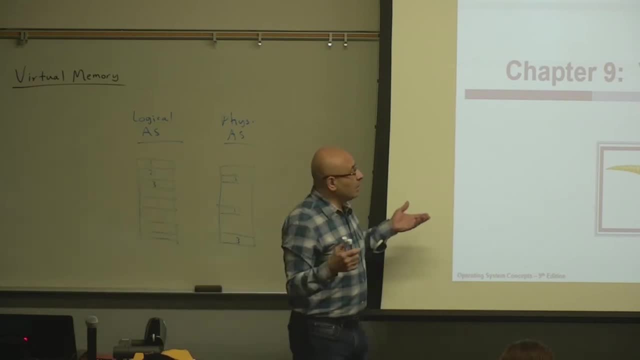 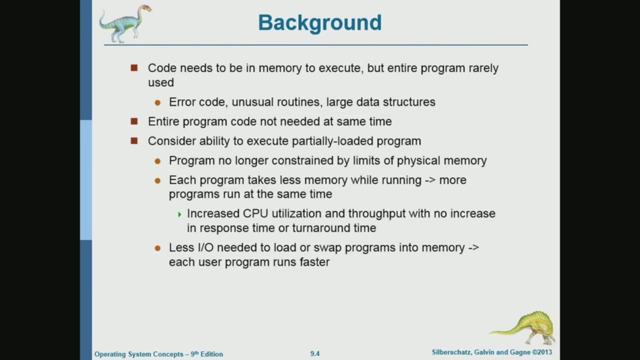 normally we don't need to load all the code and the data. So we need to load all the code and the data that constitute that program's address space. So right now I am running PowerPoint. So PowerPoint is a big application and that application 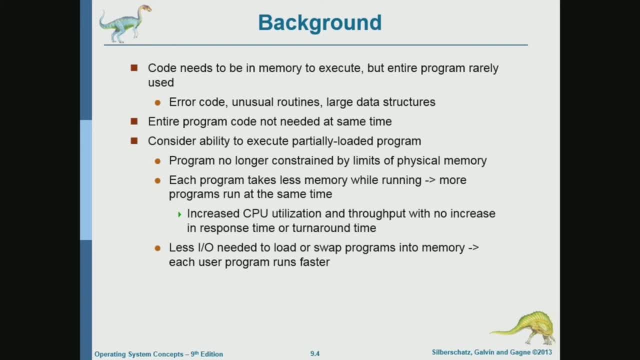 or this application has many features in it, including many features that are used for preparing these slides, Editing and preparing, and, you know, creating creating graphs and pictures and importing pictures from other applications and all of these fancy features. You know, clearly I'm not using any. 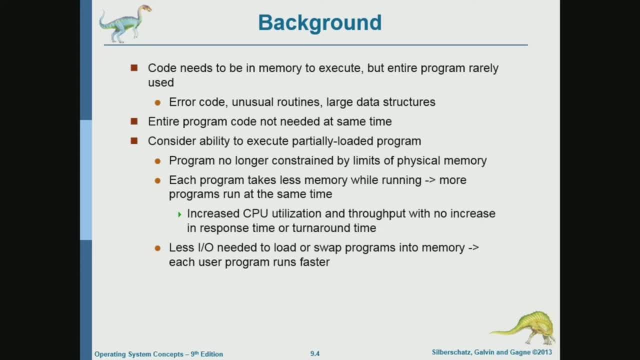 of these features at this point. At this point, I'm only using one feature of the program which is displaying these slides And, as you can imagine, this, what I'm using right now is only a small subset of the code that constitutes PowerPoint. 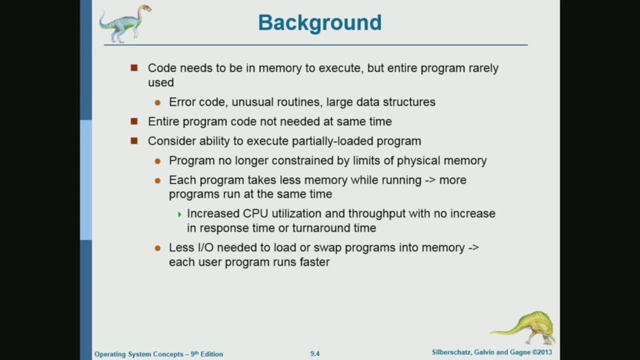 So from memory management point of view it doesn't make sense to load all the code that constitutes PowerPoint at this point It's I. I'm only using a small subset of the code and a small subset of the data. With code there is data that code uses. 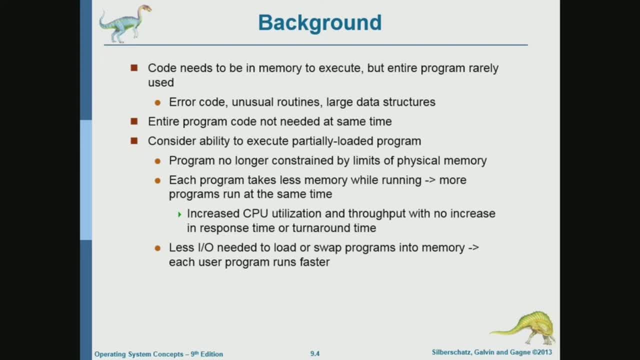 It's. it doesn't make sense to load everything. I don't need everything, I only need the subset. I only need the small subset. And that's exactly the idea of virtual memory. The idea of virtual memory is that, at any given point in time, 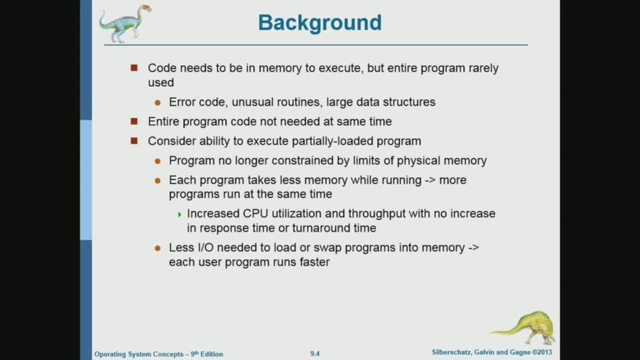 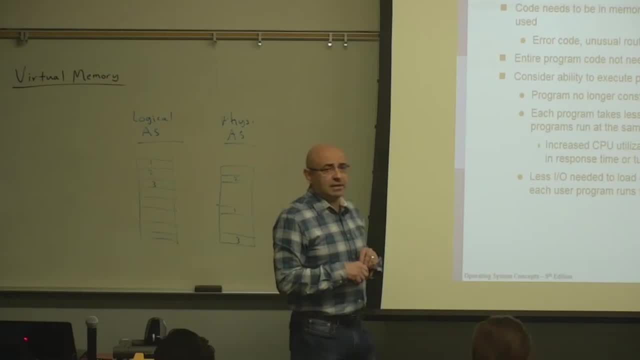 a program will only be using a small subset of its own memory. You know a small subset of the code and a small subset of the data. So, speaking in terms of pages, if I have a program with 1,000, that constitutes that you know. 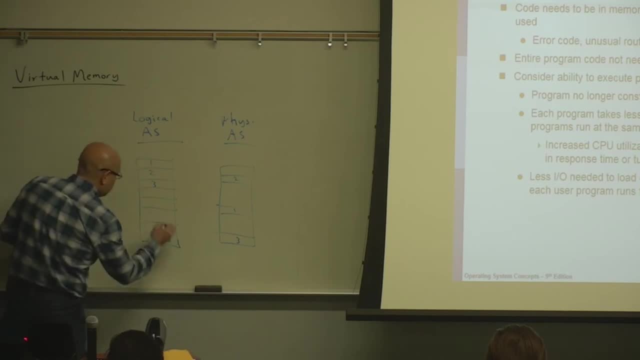 that consists of 1,000 pages at a given point in time. most likely, I'm not going to be using the 1,000 pages. I would probably be using five of them, only five pages. Like I'm using only a small number of pages. 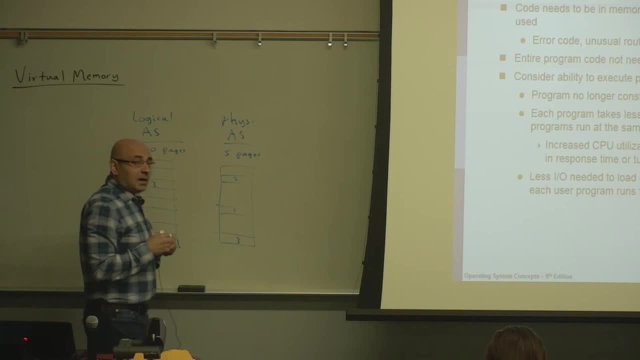 from PowerPoint at this point. So now, this is the key idea behind virtual memory. People said, okay, why do we have to load the whole thing? We only load the pages that we need, And that's the idea of demand- demand paging. 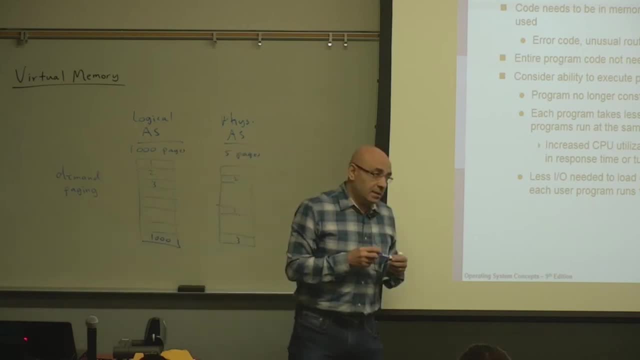 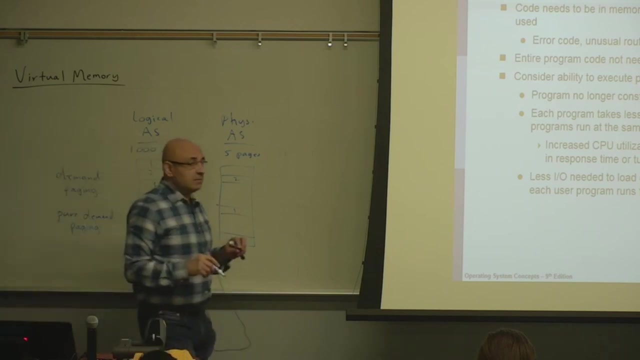 Loading pages on demand only when you need them. Now, when we talk about demand paging, the extreme case of demand paging is In pure demand paging, you strictly load pages based on demand or need, So if a page is not, you don't even consider loading a page. 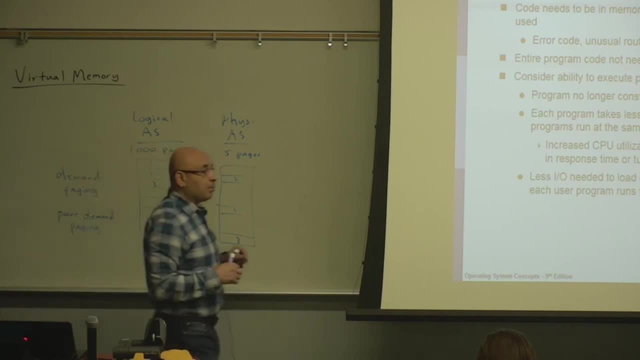 until it's requested, until the program references that page, That's pure demand paging. But what real systems actually implement is not strict or pure demand paging. It's demand paging, but the system may fetch a couple extra or a few extra pages that are not demanded. based on what? 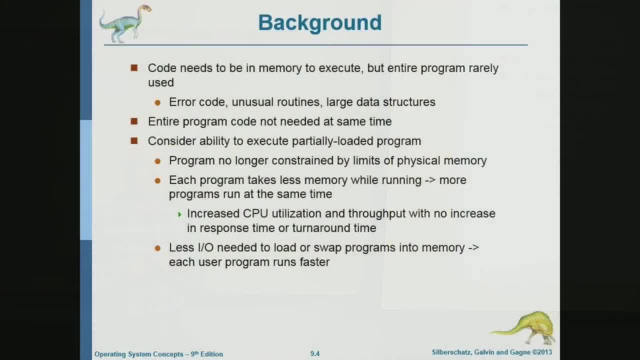 Based on what? The idea that you might need it? Yeah, And if you know if you are fetching a page, if the system is fetching one page, then you're not going to need it. So if you're fetching one page, from where will it be fetched? 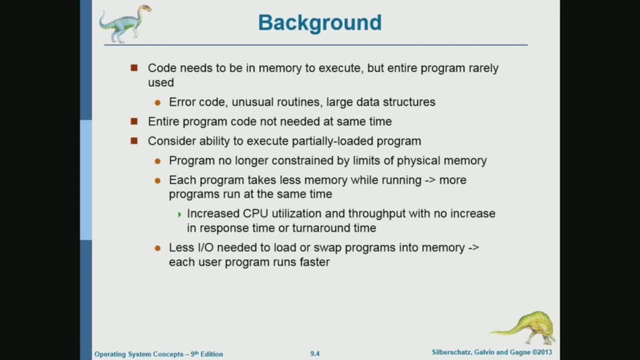 from, by the way. So when we talk about fetching, fetching from where? Yeah, Hard drive or IO? Yeah, from the hard drive. Yeah, exactly So from the disk. So in the idea, in virtual memory, is all the memory. 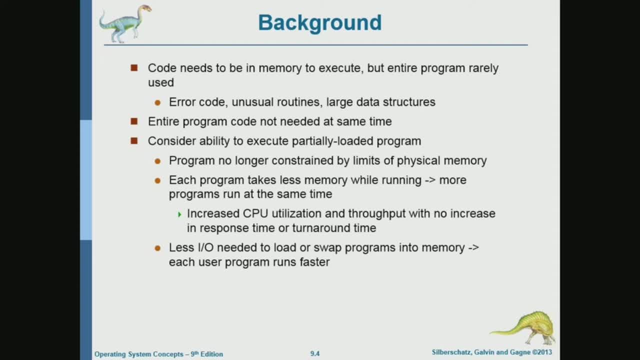 all the pages that the program needs. everything is on disk And in physical memory. I only have a subset of these pages. I have the subset that I need at this point And some systems may you know if they fetch one page. 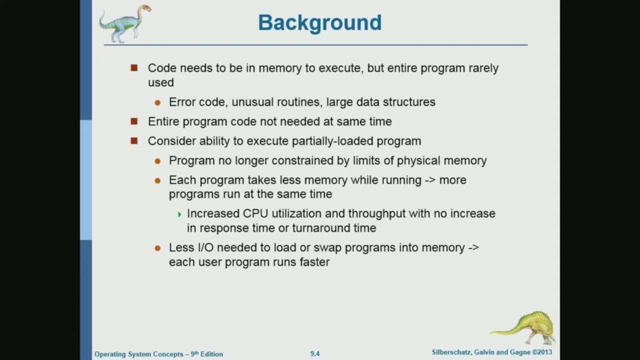 they may fetch a couple of pages that are adjacent to it. And the idea here is what, When you fetch a page and then you fetch a neighbor or two neighbors of that page, what's the idea here? Locality, Yeah, locality, exactly. 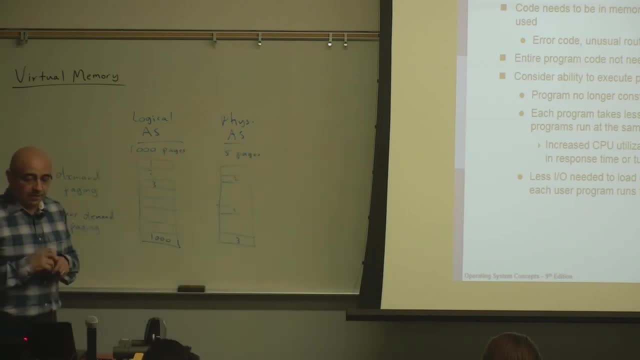 You're trying to take advantage of locality of reference because adjacent pages are likely to be referenced in the future. So now, this is the basic idea. In physical memory, I only have a subset of the pages, only that subset that I currently need. 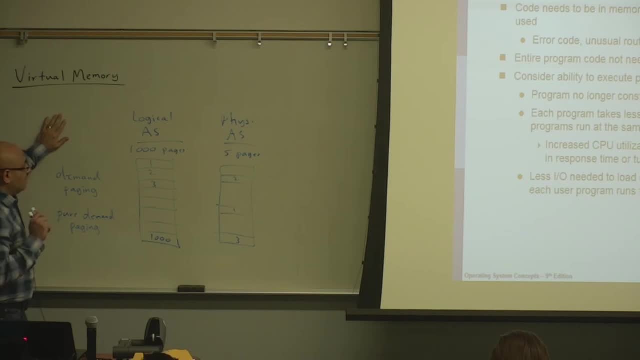 The rest of the pages are on disk. Now the advantages of this. There are two big advantages of doing this. Now, when I say that- a program with a thousand pages, I only need five pages or five frames, five physical frames, to run that program. this means that if this: 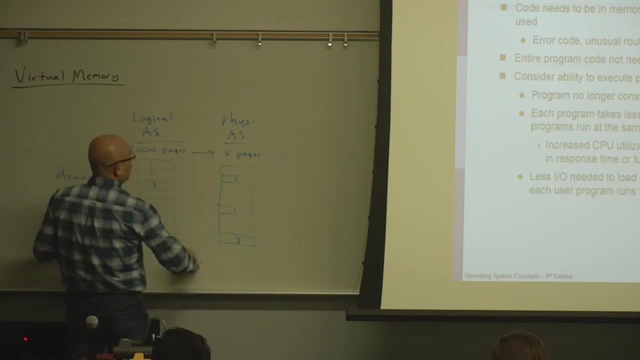 is, you know, a thousand and I only have five pages in physical memory. what I can use is, you know, I can use physical memory. I can load a lot more programs this way. If all of this, what I need to load for this program is five pages. 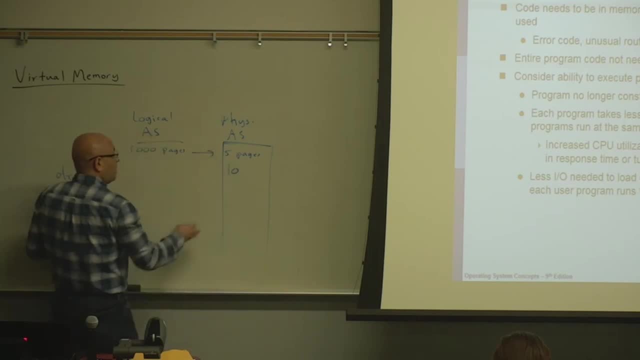 then I can load, you know, ten pages for another program and seven pages for another program and 20 pages. So this will allow me to load a lot more programs in memory. So the amount of physical memory, the physical memory that I have, doesn't have to be equal to the sum. 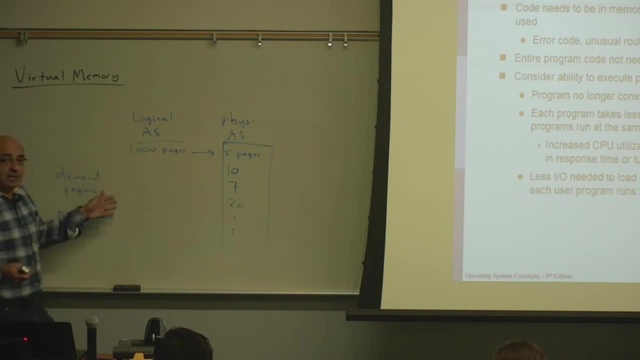 of the total sum of pages that the programs need. It has to be equal to the sum of pages that I'm using or the programs are using not the total number of pages. So I sum the five, not the thousand, which means that more programs can be loaded in memory. 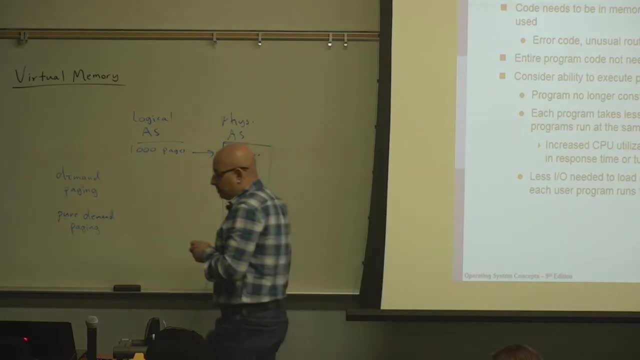 This will be the total number of pages. So this will give the system. this will allow the system to better utilize the resources, In particular better utilize the CPU. So now we can load more programs. There will be more programs in the Revit Cube. 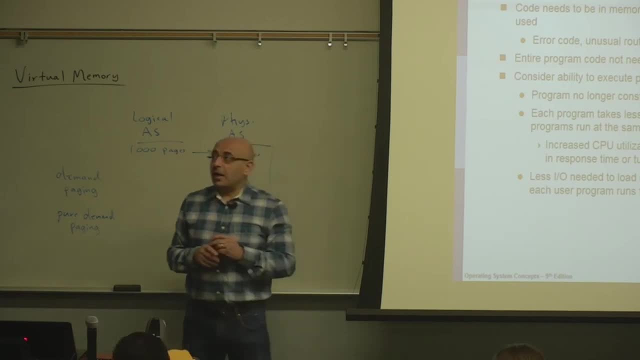 And now the scheduler. the CPU scheduler will have more options to choose from And it can better utilize. So when a process is in the waiting state, it has more options, more ready processes to select from and better utilize the CPU. 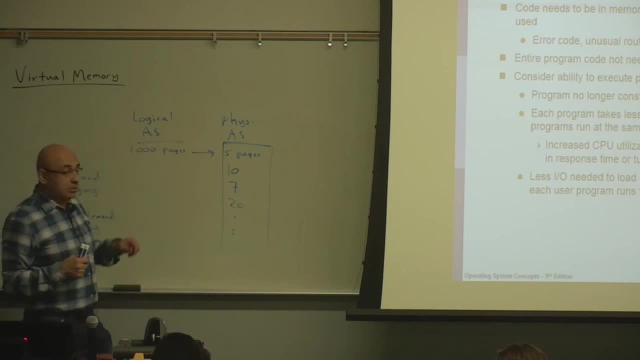 So it's. it allows the system to run more processes in parallel. It's also less disk access, because without virtual memory, if I insist on loading a thousand pages when I create the program or when I load the program, if I load a thousand pages, 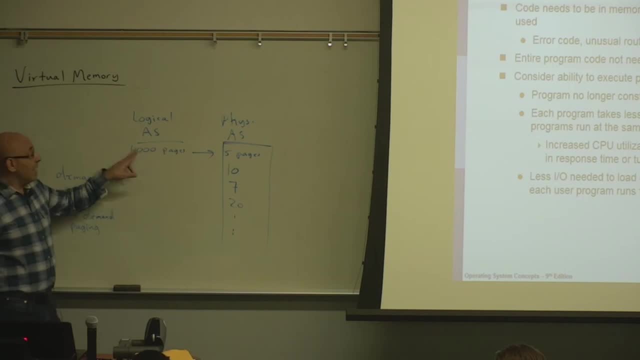 loading them. that means loading them from disk to memory And disk. the disk, as we will see, is the slowest device in the system. this means a lot of disk access, or a lot of IO, because disk is considered IO, The disk is considered IO. So 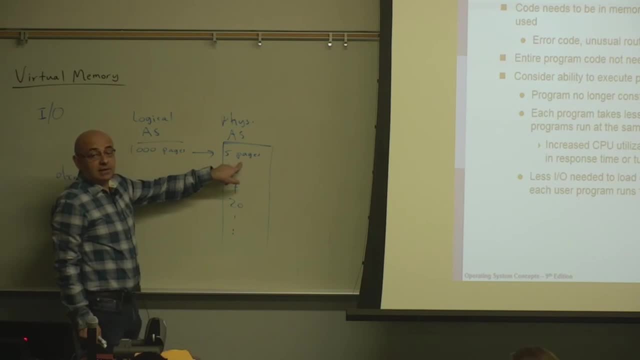 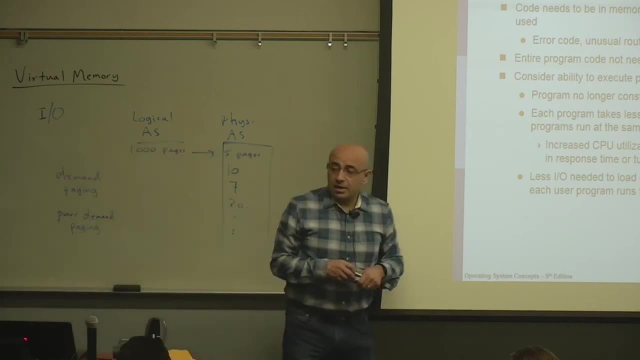 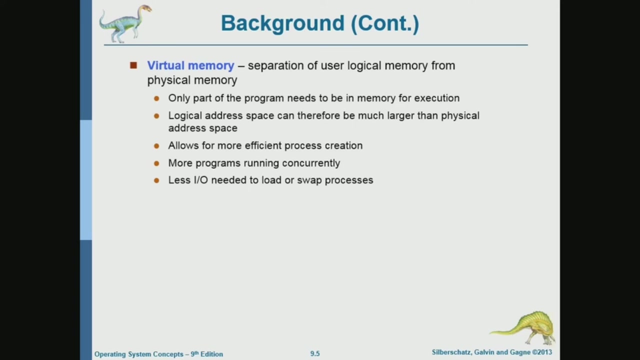 loading five pages only is going to take a lot, much less time than loading a thousand pages. So it's much less IO with virtual memory. So to summarize here: so virtual memory provides even further separation between logical and physical memory. 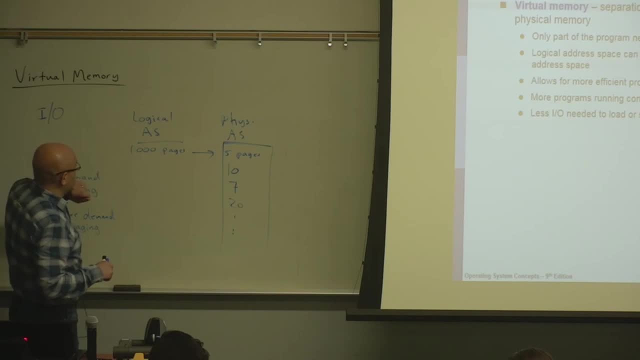 So now, not only can we use the CPU, but we can also use the CPU as a tool. So we can some pages. not only will those pages that constitute the process be scattered in memory, but many of these, these pages will not even exist in physical memory. 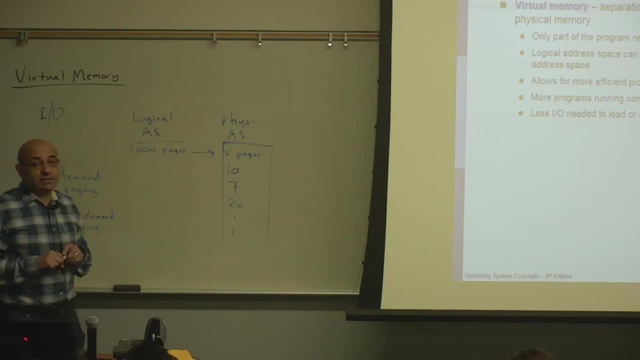 Many of the pages of a program's logical address space may not exist in physical memory at all. So now you know the difference between the logical address space and the physical address space is going to be So. the logical address space is going to be even bigger. 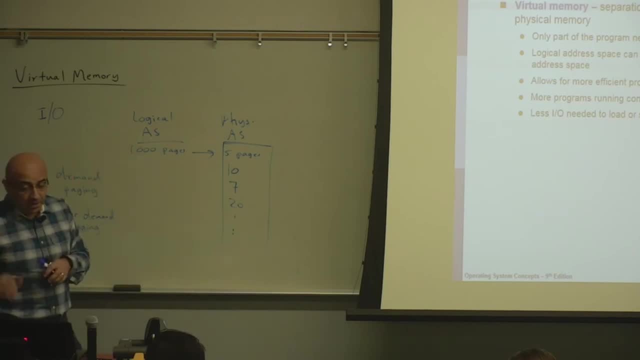 with virtual memory, because some of the pages may not be in physical memory at all And the logical address space can be bigger than the physical address space. So you know, here I have a thousand pages, Even if I have, you know, 500 pages of physical memory. 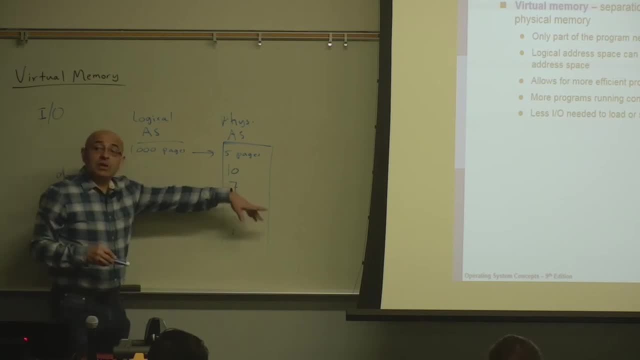 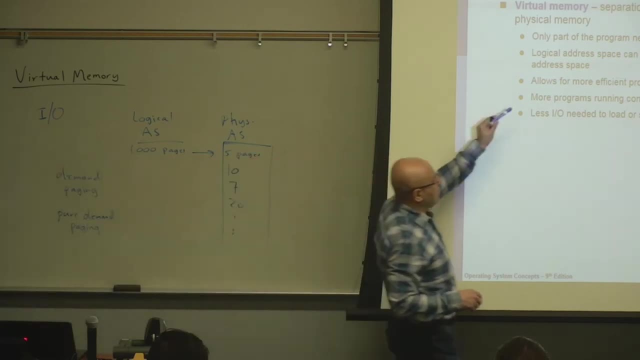 500 pages of physical memory here can be used to create a lot of memory, So I can accommodate many programs. It allows for more efficient process creation. Why? Because when I load the process I don't have to load all the pages. 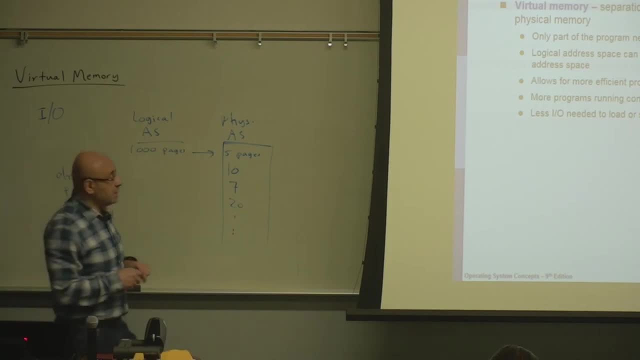 More programs running concurrently, for the reason that I have explained, that now more programs can be run into memory and the CPU scheduler will have more options. Less IO, because there is this: less disk space, disk access, sorry, less disk access. 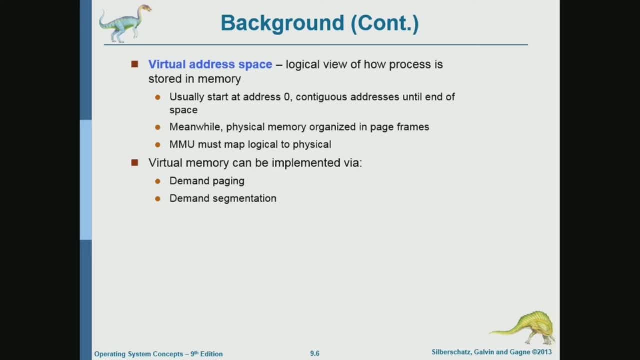 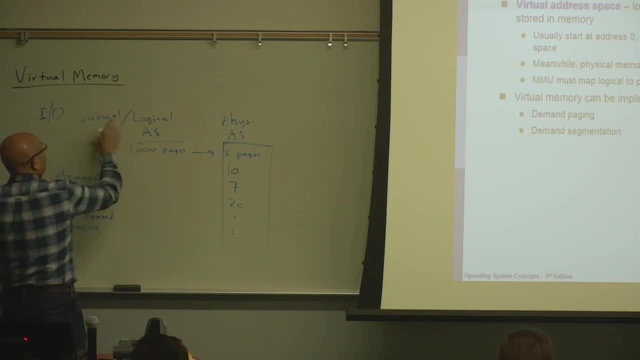 So now the logical address space. we can also call it now virtual address space. So in this chapter logical and virtual will be used. the terms logical and virtual will be used interchangeably. Okay, So now we have the notion. 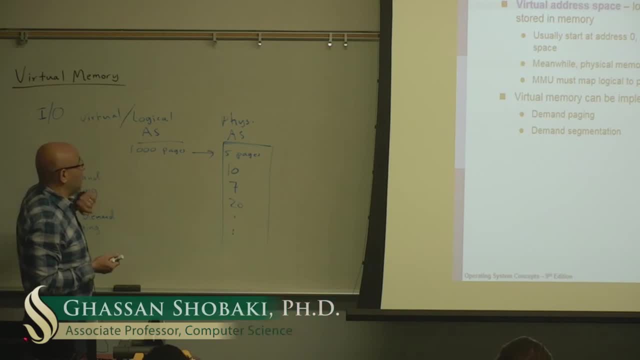 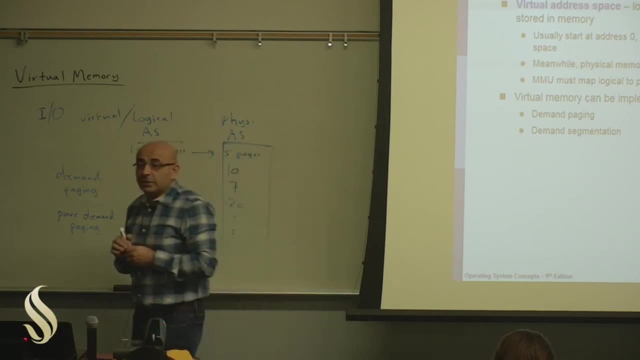 of the virtual address space. The virtual address space, which is the same as the logical address space, which will be more different than the physical address space, And we will still be using the. we will still be using the page table, which is part of the memory management unit. 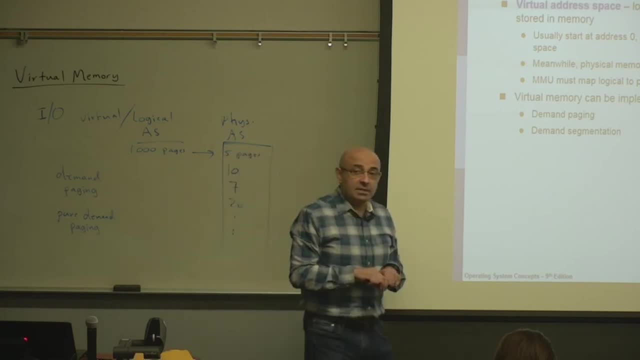 to map logical addresses into physical addresses. So in this chapter we will still be using the page table in the virtual address space. So next slide, you know, we will see the page table and what are the changes that we will have to make. 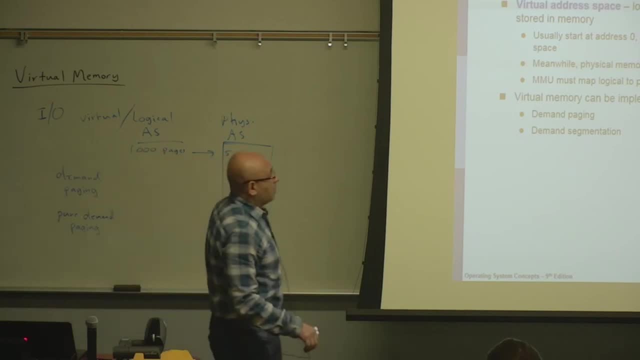 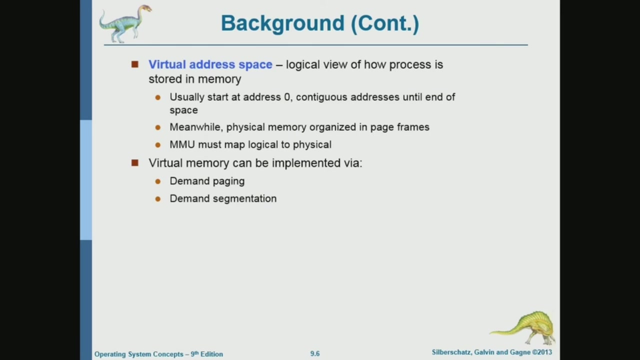 to the page table in order to make virtual memory work. So we still have page tables. In theory, you know, virtual memory can be done using demand paging and demand segmentation, but here we focus on demand paging. So the picture is like this. 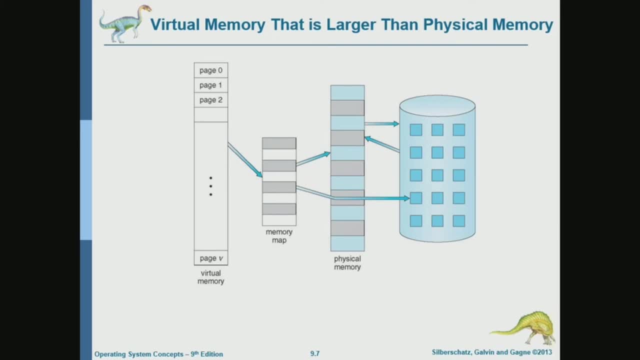 So this is the logical address space, or the virtual address space of a program, And this program has pages from zero through V. Now the memory map is the page table. you know that maps virtual memory into physical memory. In physical memory we have a subset of the pages. 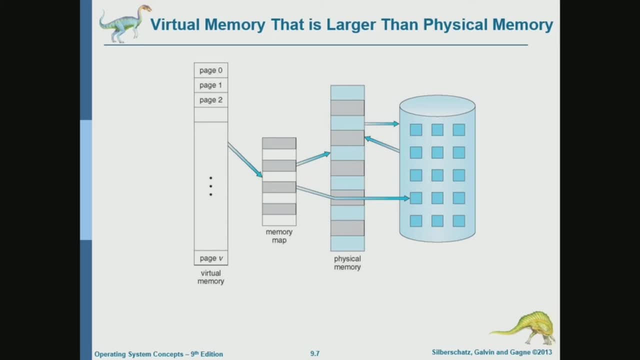 but all the pages are in this. So we will see a clearer picture in a few minutes, But for now let's look at this, the picture of virtual memory. All the pages are on this. A subset of them are in physical memory. 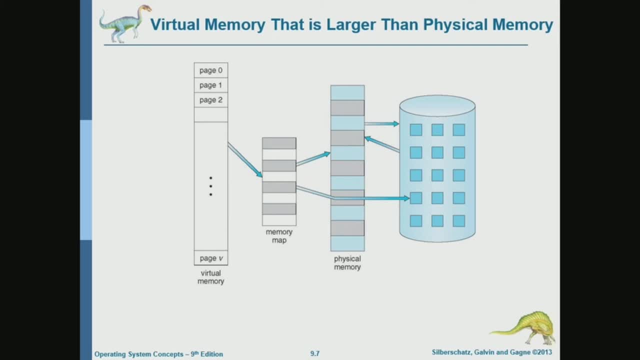 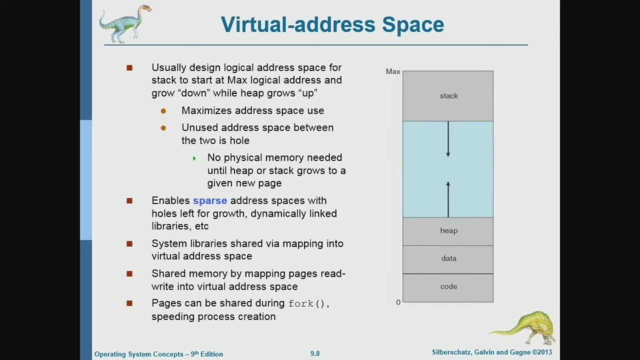 And I have a page table that maps physical, virtual to physical. So let's look at this. So that's very much the basic idea. We'll see more details later. Now, if we look at the address space of a process that consists: 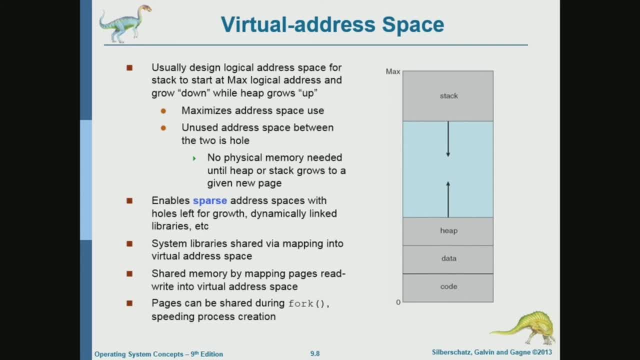 of the code segment, data segment, heap and stack, and the heap and the stack grow in different directions. Between the heap and the stack there is a hole Now in virtual memory. I don't have to allocate physical memory for this. 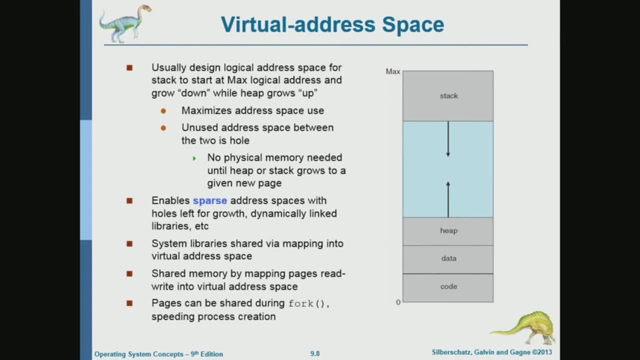 Until it's needed. You know so that when a program is running it, you know depending on what it's doing, depending on program behavior it may be, the memory that the program is using may be growing, And with virtual memory I have a lot more flexibility. 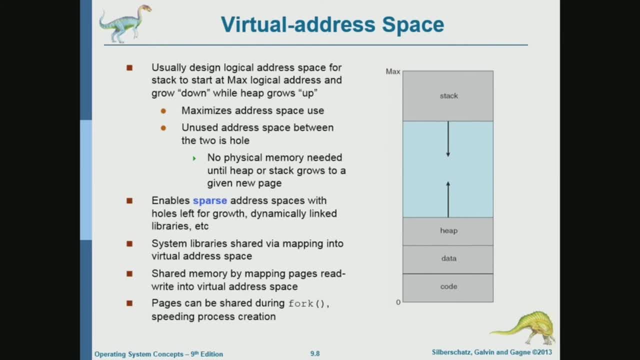 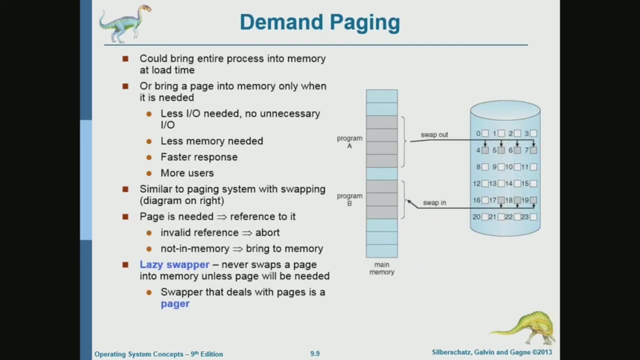 because I can allocate. I need to allocate frames only on the map, only when I need more memory, I allocate more memory. So virtual memory, virtual memory management, gives the system a lot more flexibility in handling, you know, dynamic memory allocation. 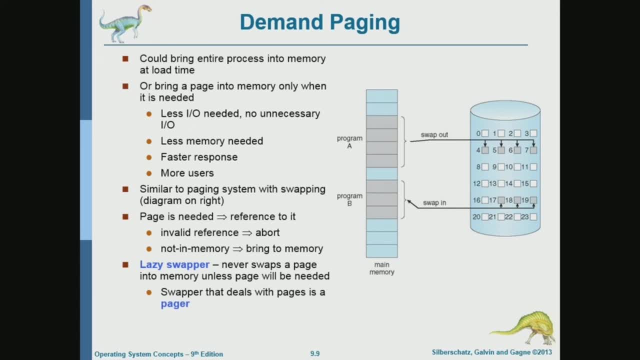 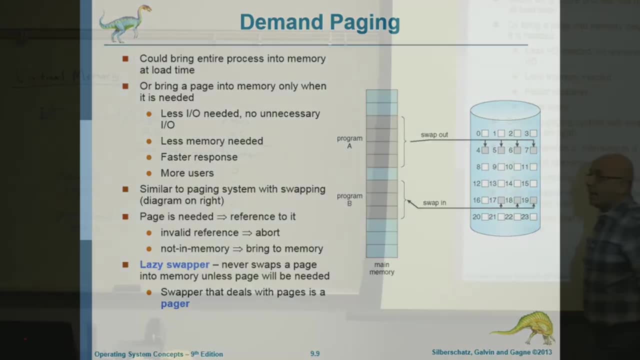 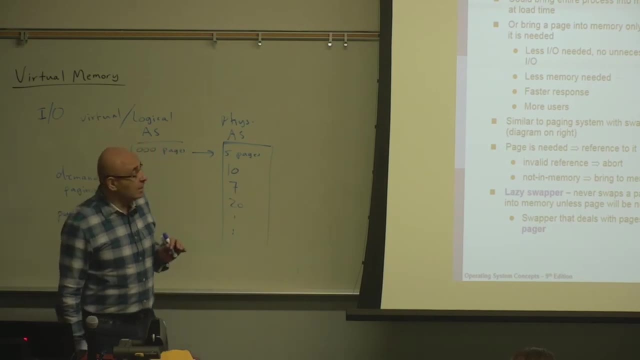 Demand paging. like I said, the idea of demand paging is fetching pages on demand. If pages are fetched strictly on demand, that's called pure demand paging. But if I fetch, if there is some kind of prediction in the system, that will fetch a few pages based on prediction or based 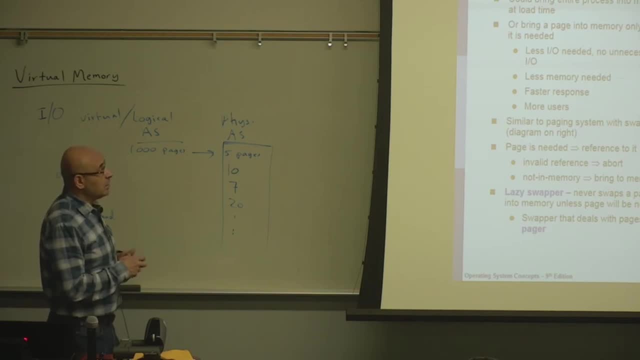 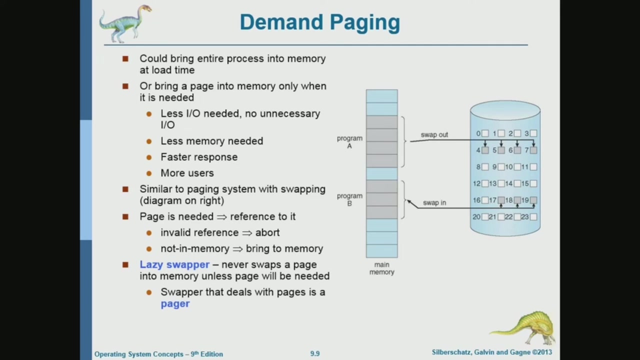 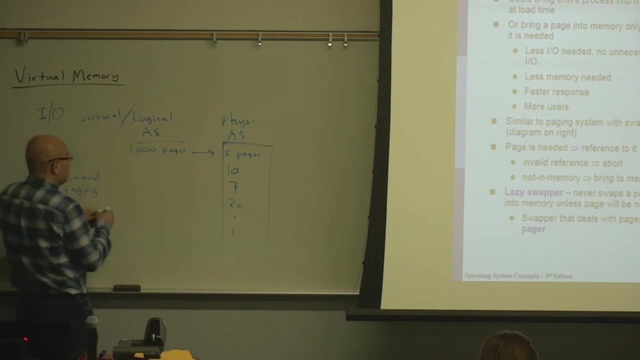 on expected future need. that will still be demand paging, but not pure demand paging. When the program references a page first we will check on that reference if it's valid or invalid. So if a program has 1,000 pages and it references page 7,000,. 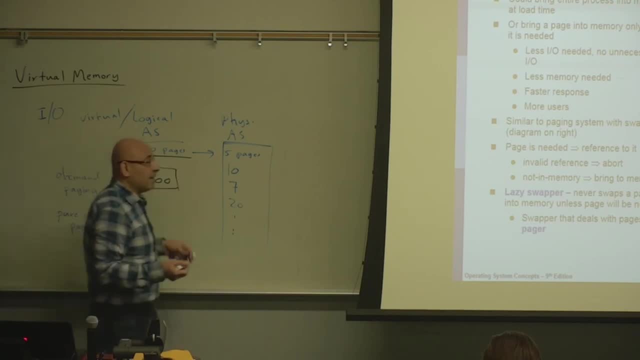 so page 7,000 doesn't exist, So that's an invalid access. But if it's referencing something valid, something between the two, then it's valid. But if it's referencing something between, you know, page 0 to page 999, that's in the valid range. 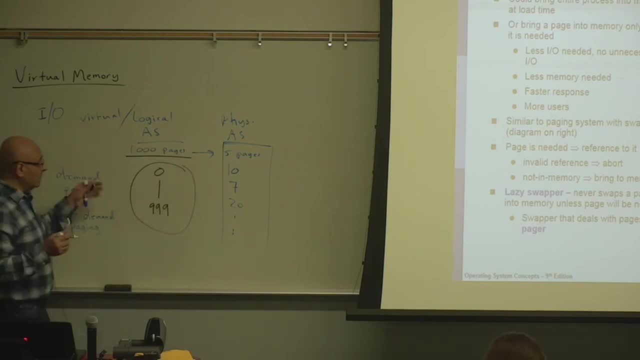 But not all of these are going to be in physical memory, So we will need a way of checking whether that page that is being referenced is in physical memory or not. If it's in physical memory, we'll access it like normal. If it's not, then the system will have to fetch it from this. 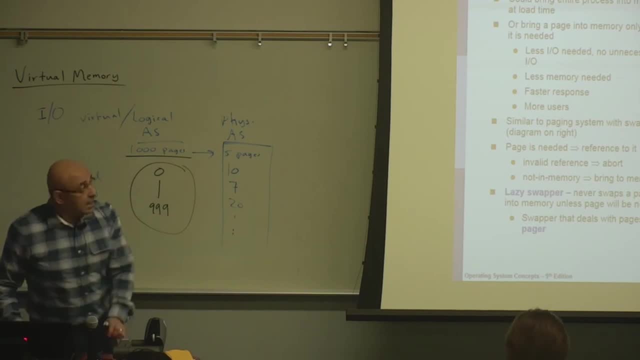 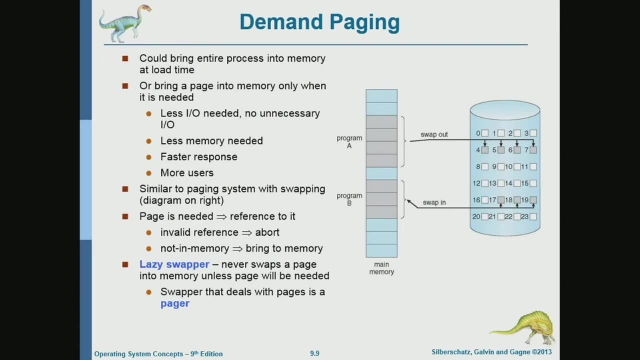 and load it into physical memory. Now, this is very important, You know. this shows you swapping of a whole program In virtual memory. this is not what we do. We don't swap a whole program, We swap a page. So it's basically what virtual memory is about is doing the 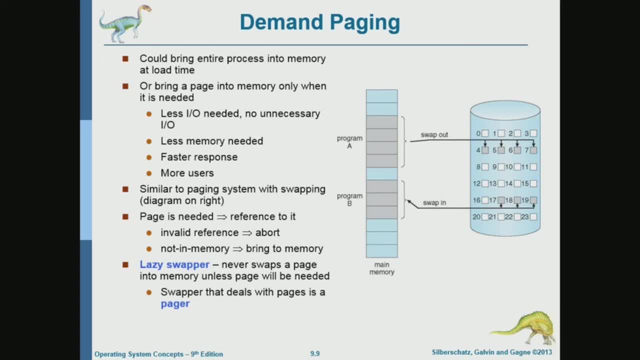 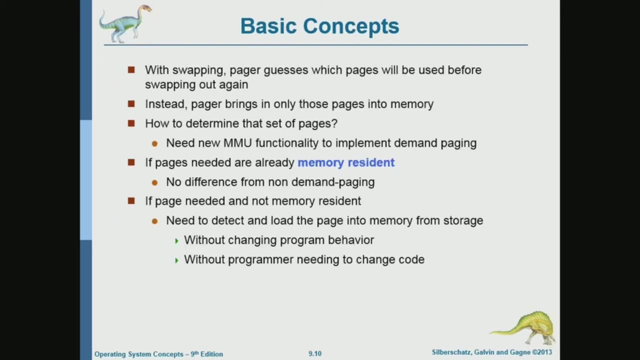 swapping in and swapping out of at the page level, rather than the whole address space. Now, in order to you know, in order to you know, to implement this, we need a way of detecting whether the page that is requested by a program is in physical memory or not. 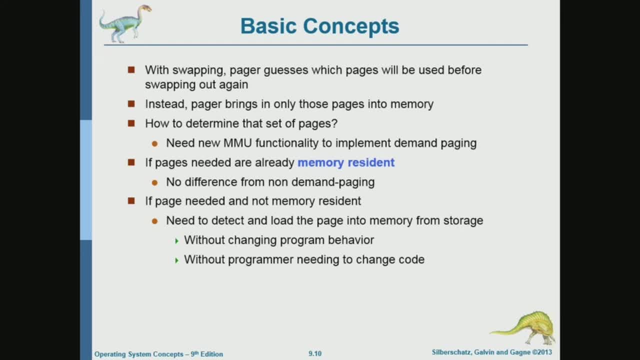 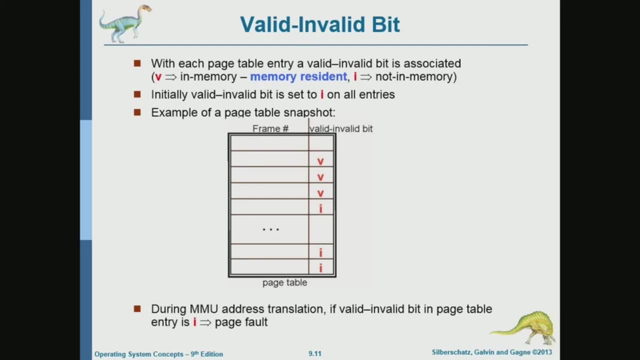 And that mechanism is the valid invalid bit that is added to the page table. So now in the page table there is an additional bit that is added to each page, Each frame. Yeah, So there is an additional bit that indicates whether that frame is in physical memory. 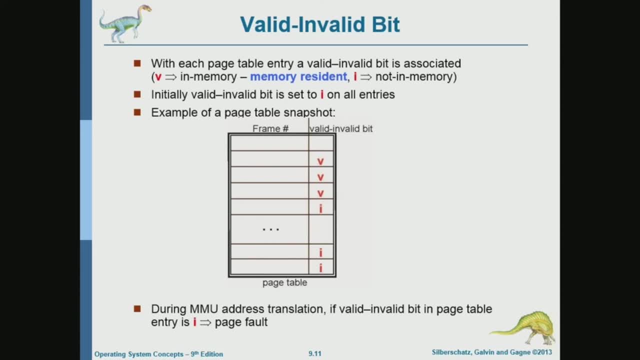 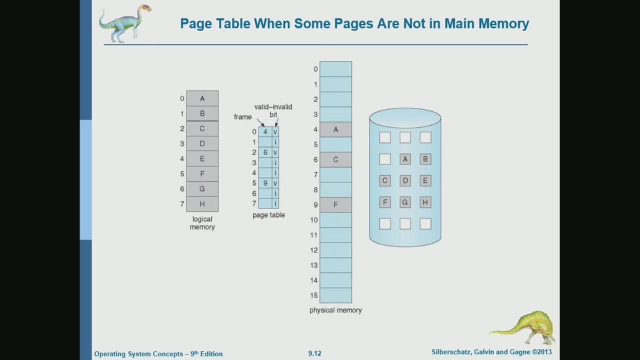 or not. So V means valid, It's in physical memory. I means invalid. It's not in physical memory, It's on disk. So let's see how this is used. I think this is a very good picture that shows you know how virtual memory works. 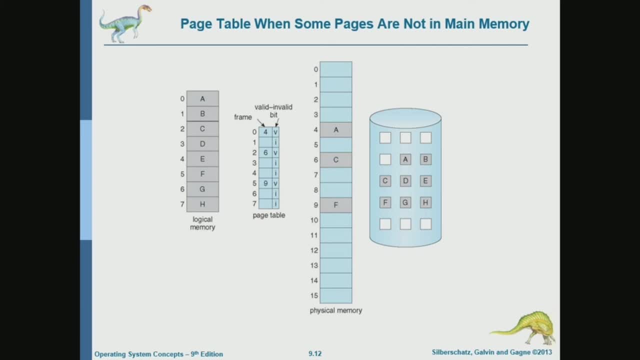 So we have logical memory. So we have, in this example, a program that consists of eight pages, zero through seven, And this is physical memory, And this is the disk. Now, on disk we have all pages. So everything is on disk: A, B, C, D, E, F, G, All. 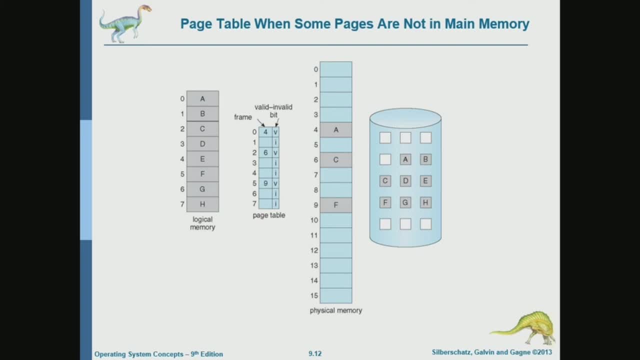 of them are on disk, Only a subset of them are in physical memory. So I have page zero, which is in frame four, is in physical memory, So I have the valid bit set. I have page two, which is in frame six, in physical memory. 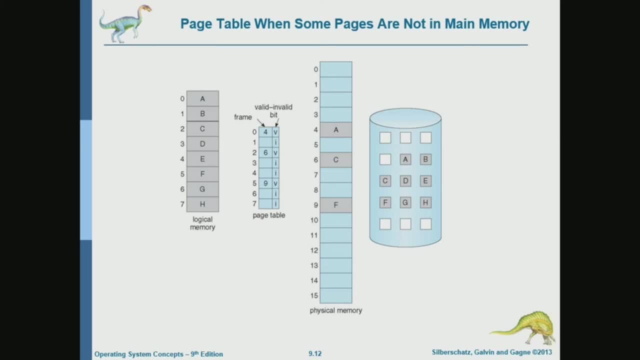 And the valid bit is set. And I have page five, which is in frame nine, And the valid bit is set. Now, for the rest of the pages, the valid bit is reset, or it's I here indicating that it's not in physical memory? 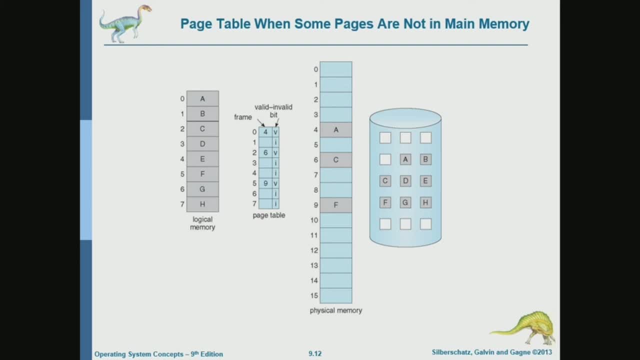 So now, when we access, when the program references a page, if it references page zero, it's in physical memory, So this is a normal access and it will just access that page. But what if the program attempts to reference page one? 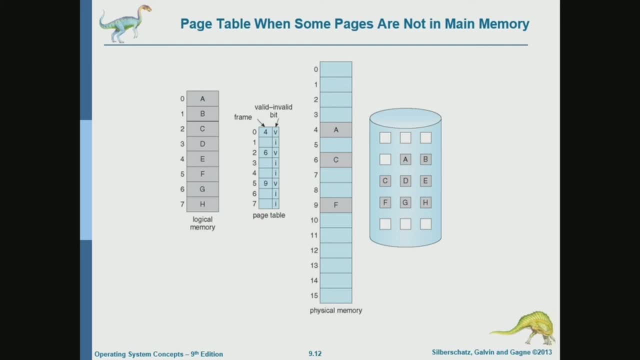 So the program, which is not in physical memory, it's on disk. Now we need to fetch that page from disk. Now who will be doing that fetching of the page from disk to memory? Will it be the application or the system? 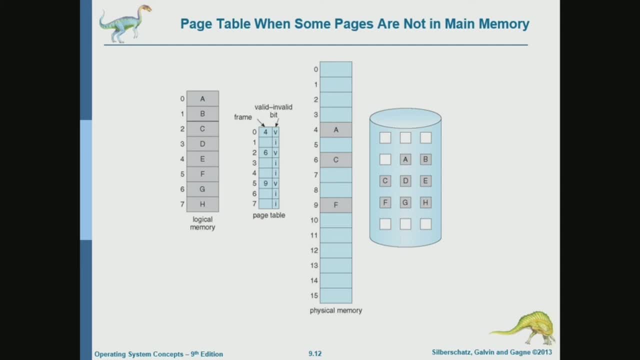 System- Yes, it's going to be the system. So we have to give control to the system somehow, And that's why implementing virtual memory requires hardware support. Okay So, hardware support by having one kind of exception, or an exception or an interrupt that will give control. 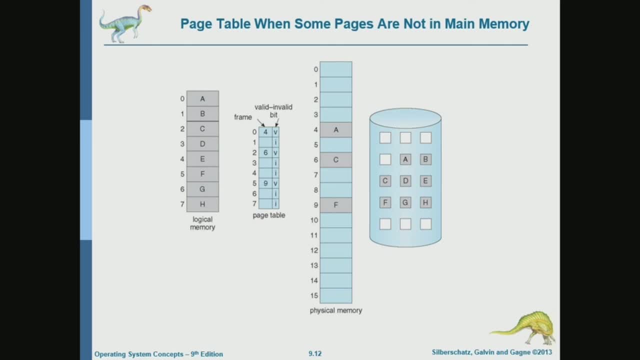 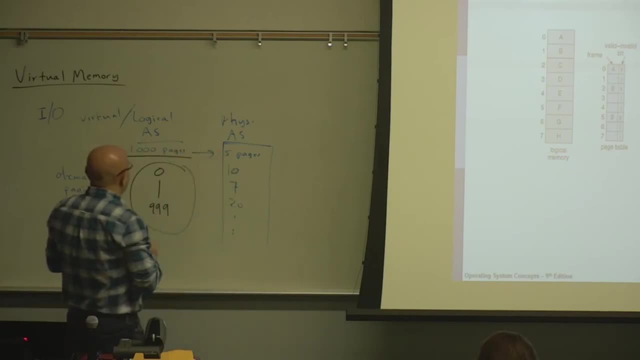 to the system when the program makes access to an invalid page. So and then we have to make sure that the program is all in physical memory, and this is what we call a page fault. By the way, we will in the next lecture. 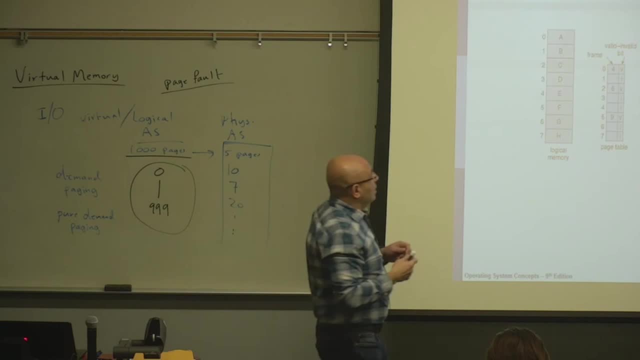 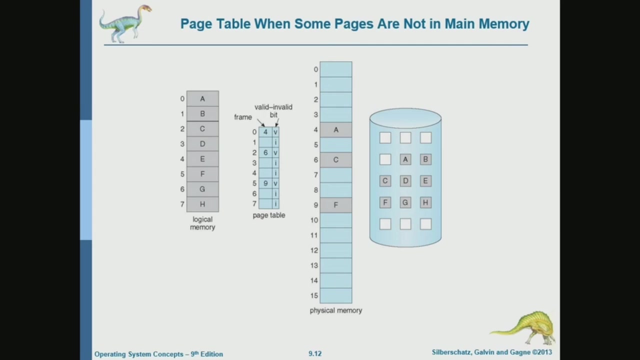 we will learn more details about page faults, But for now the concept is a page fault is when a program attempts to access a page that is not in physical memory, like page one in this example. That will result in a page fault. A page fault is an exception and that will give control. 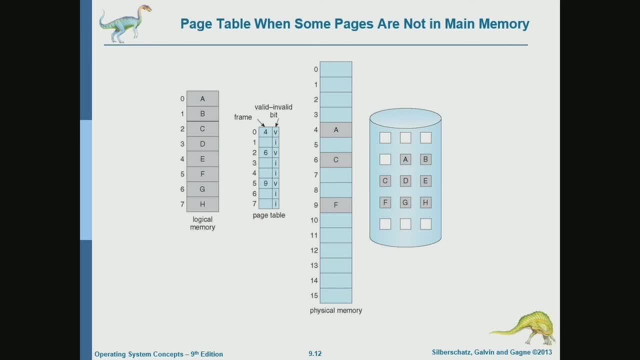 to the operating system. The operating system now will be in charge and it will load that requested page like page one in this case. It will load it from disk into physical memory and it will update the corresponding page table entry to reflect that this page is now valid. 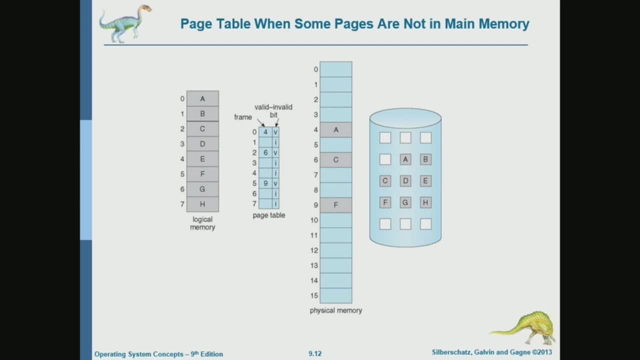 It's in physical memory And do you think that that page fault is a slow or a fast process? How fast or slow do you think page fault handling will be? It might be kind of slow because you have to go all the way to the disk to grab it. 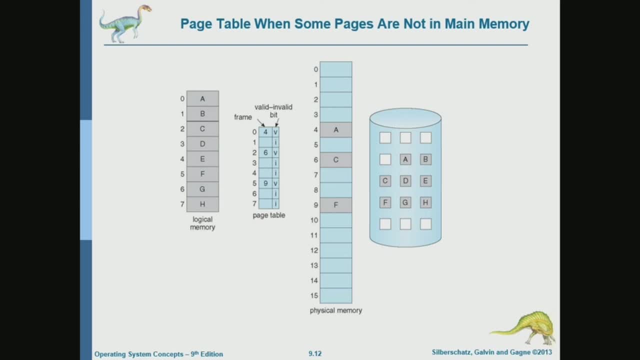 Yeah, exactly, You have to go to the disk and the disk is very slow. Keep in mind that the disk is very slow. As we will see. it's orders of magnitude slower than memory. So going to the disk is very slow. 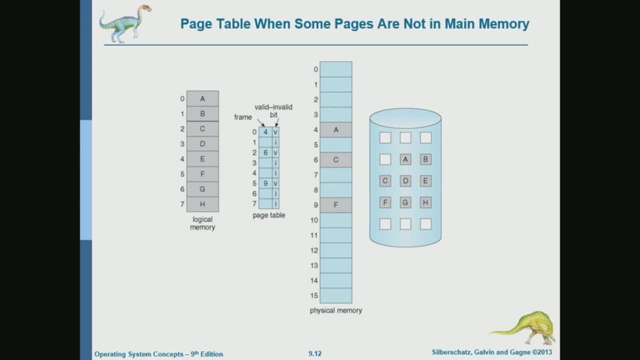 It's going to take a lot of time, So that's why you know. that's the good thing about giving this to the, this responsibility to the operating system. The operating system will handle the page fault and it will send a request to the disk to load that page. 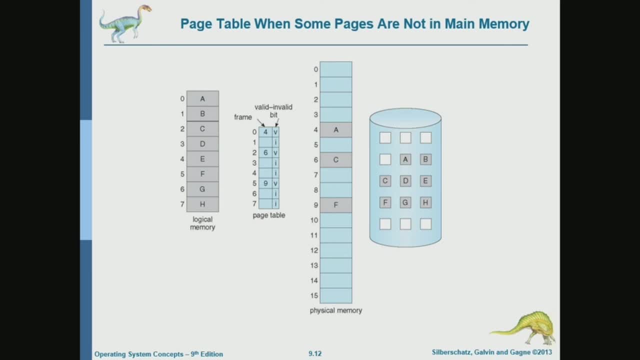 But in the meanwhile it will give the CPU to another process. So while one process is waiting for a page fault or for page fault handling, the system can give the CPU to other processes. Now you know page faults. we'll talk about page faults. 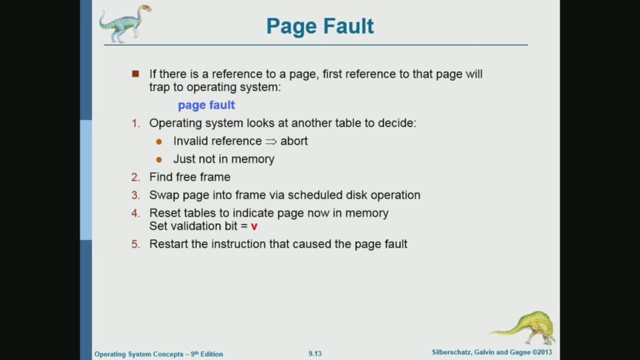 in detail next time. but the idea now is: we know, now it's clear to us that page fault handling is very slow. Now how does virtual memory work then? Why does Virtual memory work, you know, effective in real programs? 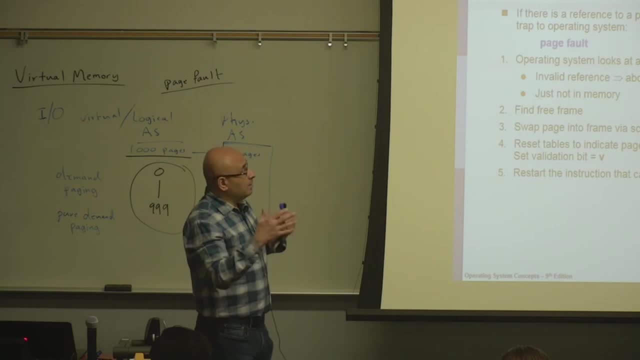 The page fault is too slow or the page fault. handling takes a lot of time and whenever a program references a page that is not in physical memory, we'll have to take a page fault, give control to the operating system and the operating system fetches that page fault. 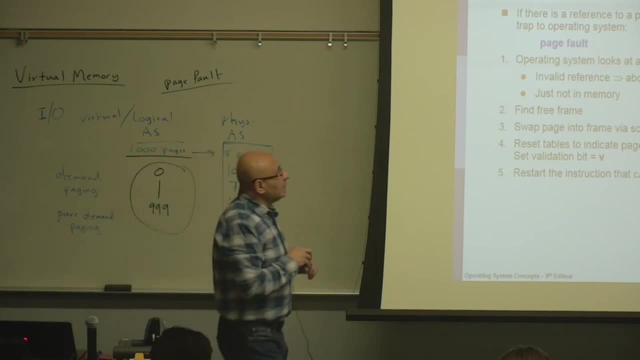 Right, Yes, Yes, It fetches that page from disk to memory. It sounds like there will be lots of time that programs will be standing waiting for the system to handle a page fault. So it sounds like this is going to slow programs considerable. 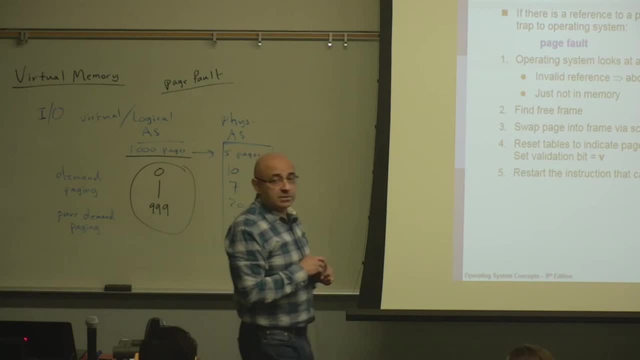 Now the question is: why doesn't this slow programs considerable? Seems like they're probably really good at it, So maybe 99% of the time you won't ever have a page fault. If you do, you just run out of time. 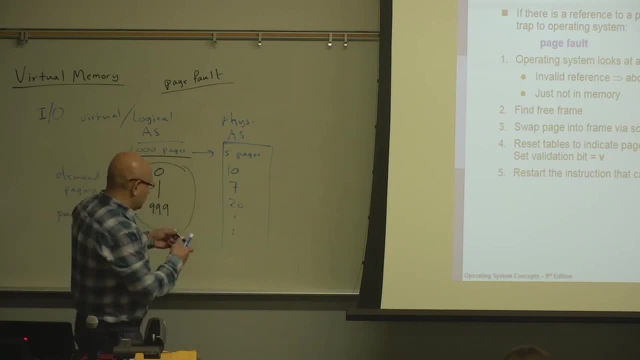 So you're saying 99% of the time, or most of the time, there will be no page fault. Why? Because it already has loaded all of the pages that are around that he said it was already working on. So it already has extra pages that you'll probably use.